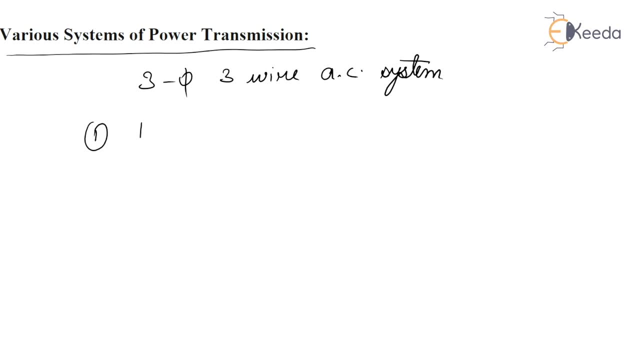 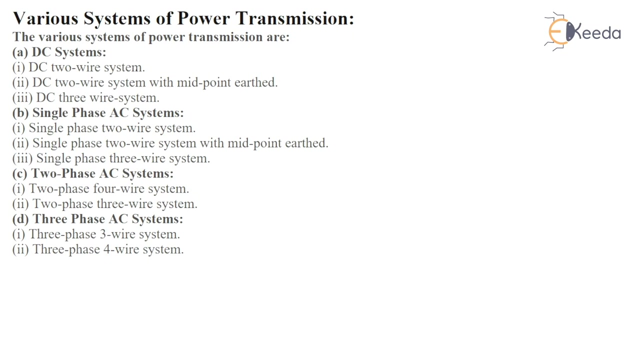 The different possible systems of transmission are DC system, single-phase AC system, 2-phase AC system and 3-phase AC system. These systems are again characterized into DC system, characterized into 3, DC 2-wire system, DC 2-wire system with midpoint earthen DC 3-wire system. 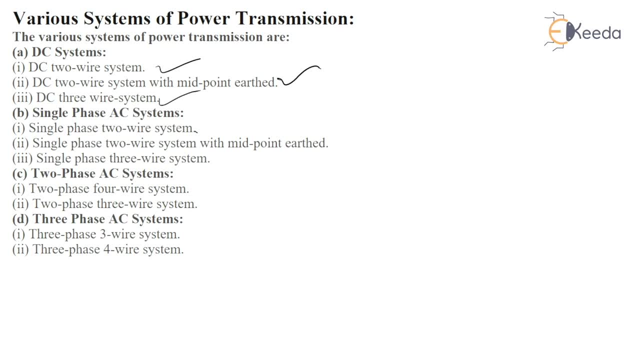 Single-phase AC system is again characterized into 3, single-phase 2-wire system. single-phase 2-wire system with midpoint earthen. single-phase 3-wire system. 2-phase AC system is characterized into 2, 2-phase 4-wire system. 2-phase 3-wire system. 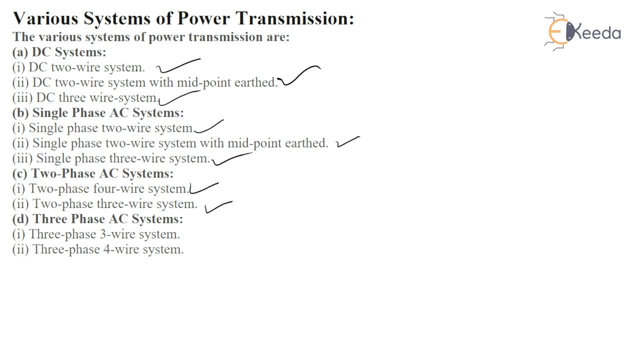 3-phase AC system is characterized into 2, 3-phase 3-wire system, 3-phase 4-wire system. This 3-phase 3-wire AC system is universally adopted for transmission of electric power. From these possible systems of power transmission, it is difficult to say which is the best system. 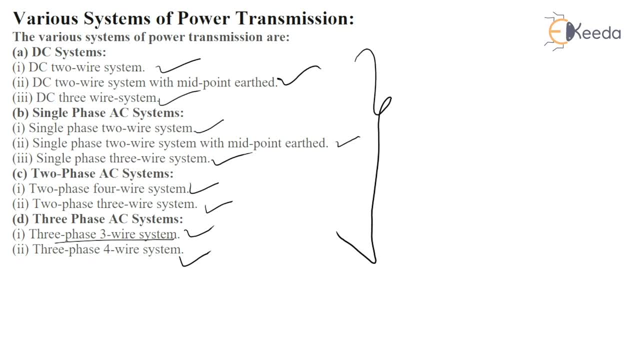 until and unless some methods comparison is adopted. Now, cost of conductor is one of the important charge in a system. Obviously, best system for transmission of power is that for which volume of conductor material required is minimum. Therefore, the volume of conductor material required forms a basic comparison between different systems. 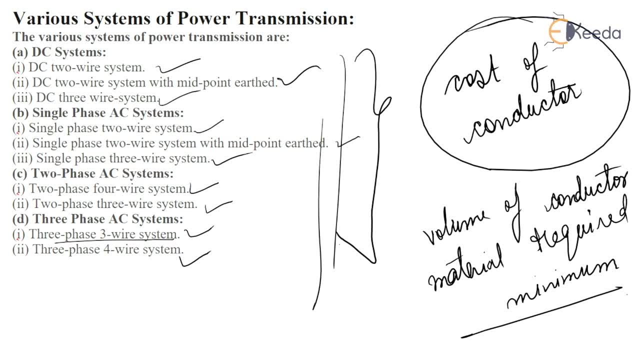 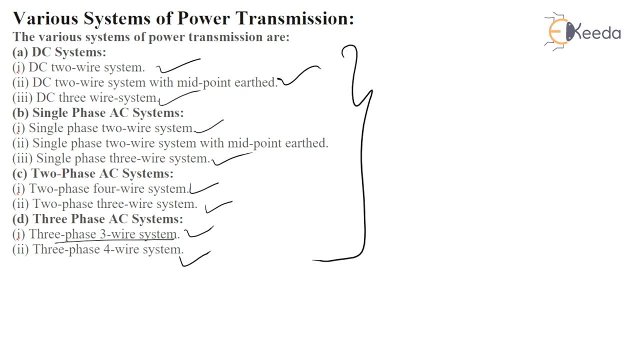 Now let us calculate the volume of conductor material required From these possible systems of power transmission. it is difficult to say which is the best system until and unless some methods of comparison is adopted Now. cost of conductor material is one of the important charges in a system. 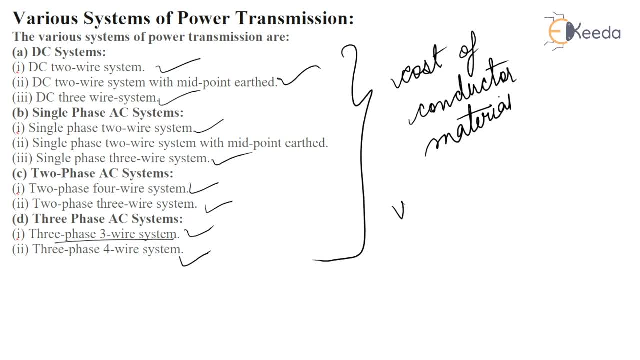 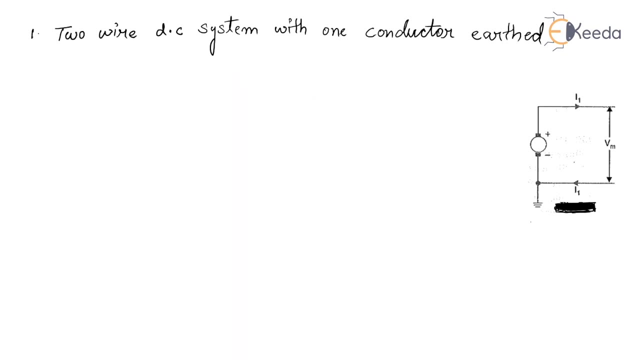 Obviously best system for transmission of power is that for which volume of conductor is minimum. Therefore, volume of conductor material required forms a basic comparison between different systems. Now, volume of conductor material required forms a basic comparison between different systems. So first calculate for DC system. 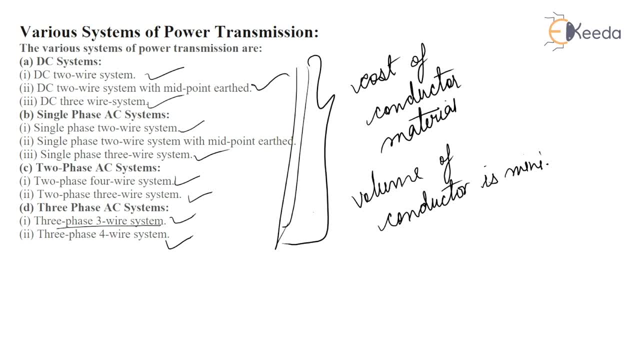 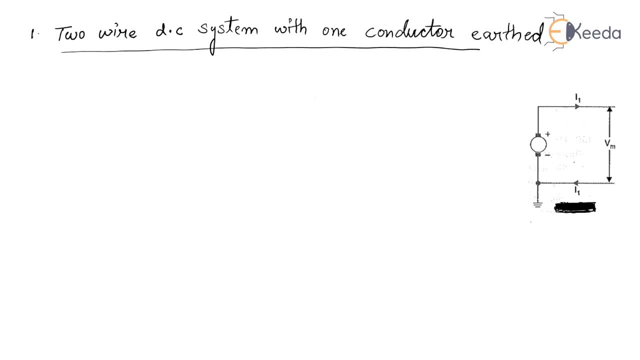 First one is DC system for 2-wire system. 2-wire DC system with one conductor is minimum. So first one is DC system for 2-wire system. So first one is DC system for 2-wire. DC system with one conductor is minimum. 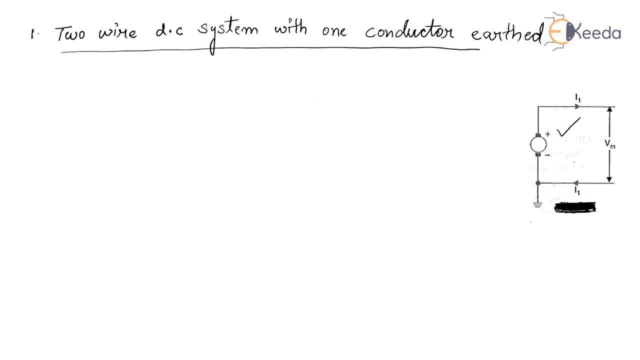 In 2-wire DC system. one is the outgoing or positive wire, Second one is the return or negative wire. Load is connected between the two wires. Maximum voltage between conductor is Vm. Power to be transmitted is P. Therefore load current is equal to power upon maximum voltage. 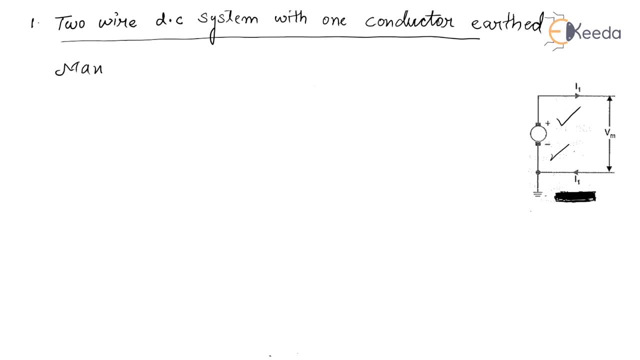 So maximum voltage between conductor is Vm and power to be transmitted is P. Therefore, load current is equal to power upon maximum voltage. Therefore, load current is equal to power upon maximum voltage. Therefore, load current is equal to power upon maximum voltage. 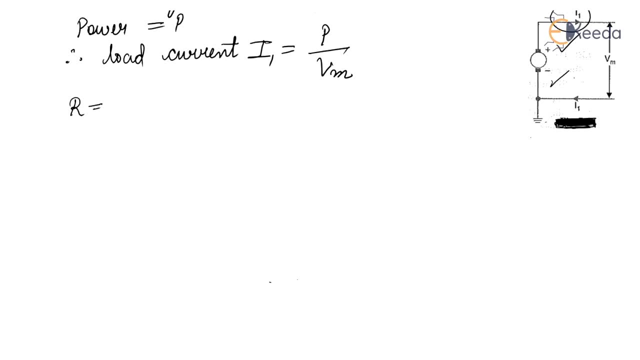 And P is the present current Vm and R is the Lock current. This P- Vermont current are receive as layer año for our function to function. that is working for ECM-. if Sayныйவ is a resistance of each line conductor, then R is equal to rho a1.. can stand. if R is the resistance of each line conductor, then R equals rho L by a1, where a is the exsection of the conductor in the area of the exception of the conductor Can stand. if R is a resistance of each line conductor, then R is equal to rho L by a1, where a is the exception of the conductor. area of acceleration of conductor. 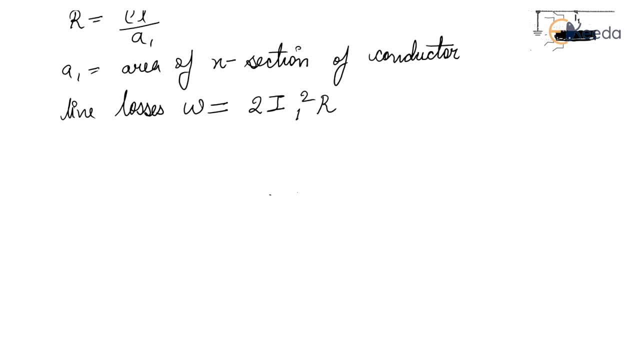 L MsPW of conductor to x section of the conductor Line losses for 2- drive between two fierimetry of circuit where I is P upon maximum voltage and R is Rho L by A. Put the value of I and R powered upon maximum voltage into Rho L by A. 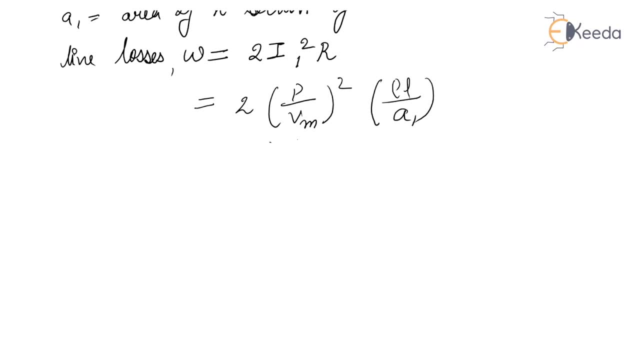 We have to find out the volume of the conductor material required for 2-wire DC system. So volume of conductor material required for 2-wire DC system is 2 area into length, So we have to find out the area. 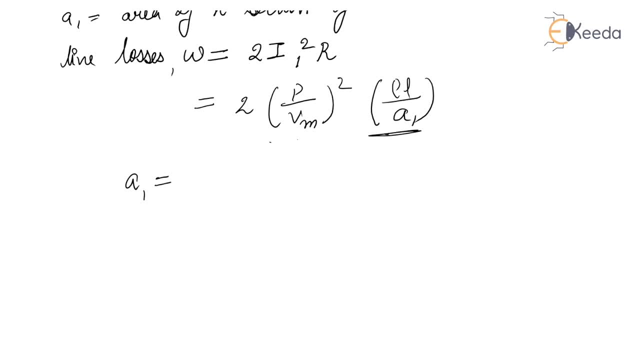 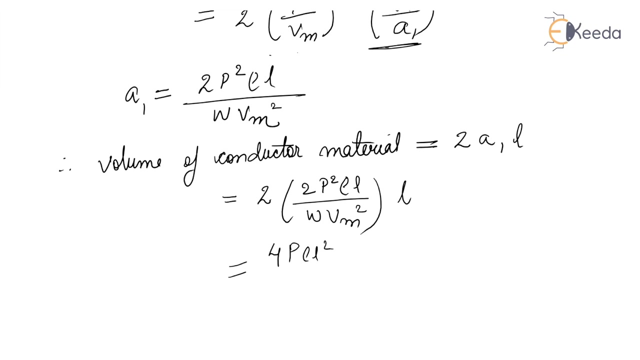 From this equation, area is equals to. therefore, volume of conductor material required for 2-wire DC system is 2 area into length. where area is, this is equals to 4 P square, Rho L square upon W Vm square. Let's say this value is k. 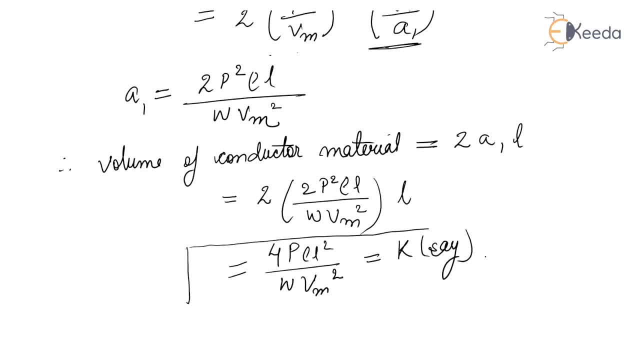 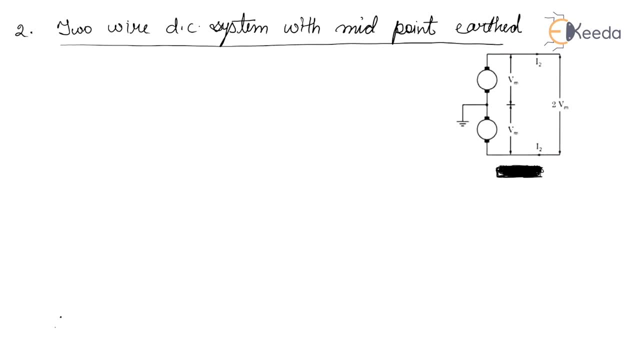 This is the volume of conductor material required for 2-wire DC system. Now the volume of conductor material required for 2-wire DC system with midpoint earth DC. 2-wire system with midpoint earth. Maximum voltage between any conductor is Vm. 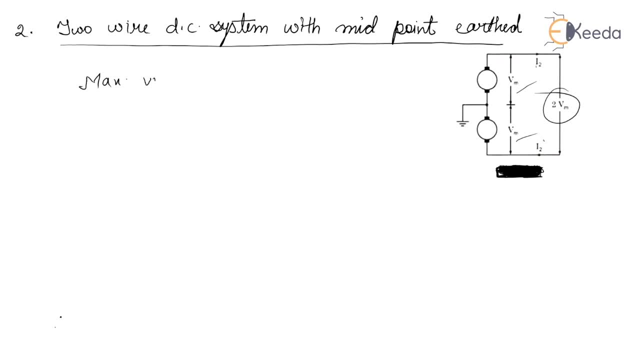 So the maximum voltage between conductor is 2 Vm. Power to transmitted is equals to P. Therefore load current is equals to power upon maximum voltage. Now again, if R is the resistance of each line conductor, then R is equals to Rho L. 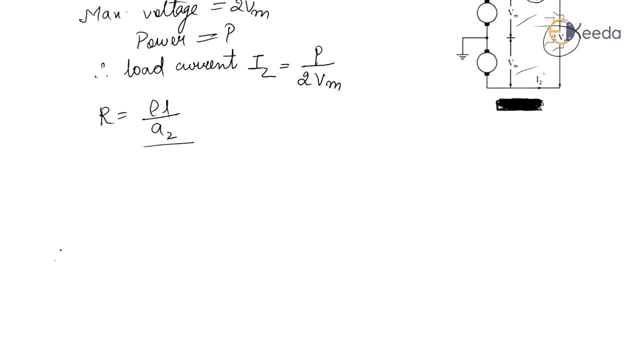 upon A2.. Where A is the area of the x-section of the conductor, So this is equal to Rho L upon A2.. Where A is the area of the x-section of the conductor, So this is equal to Rho L upon A2.. 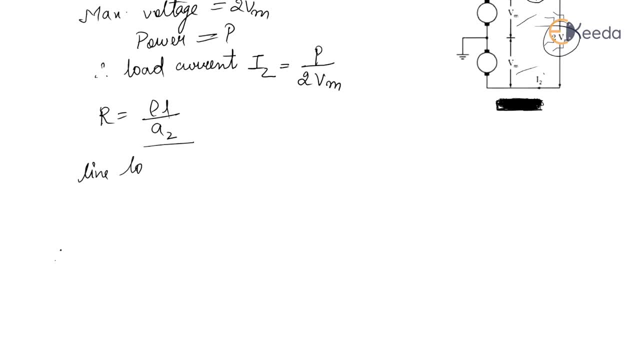 So this is equal to Rho L upon A2.. Then line loss is A equals to 2. I square R, Where I is power upon 2 Vm and R is Rho L upon A. Put the value of I and R. 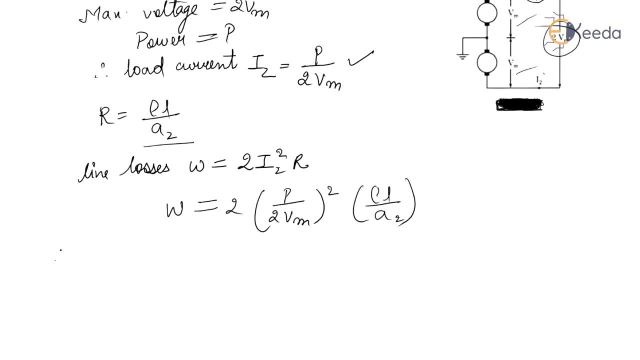 For volume of conductor material required for 2-wire DC system with midpoint earth end. the volume of conductor material required is 2 area into length. So from this equation we have to find out the area. So area is equals to 4 Vm square W. It is equals to P square Rho L upon 2 Vm square. 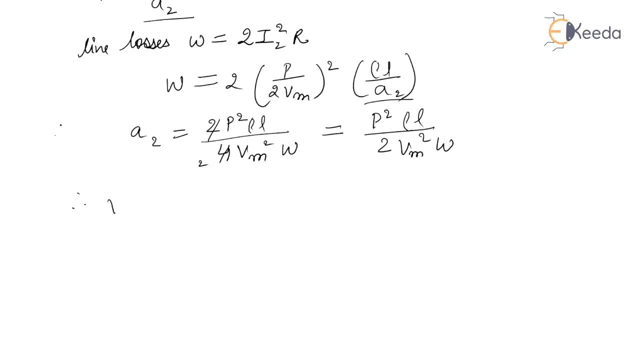 W. Therefore, volume of conductor material required is equal to 2 Rho L into length. Put the value of area, It is equal to P square Rho L square upon. Vm square into W Now 4 P Rho L square upon. 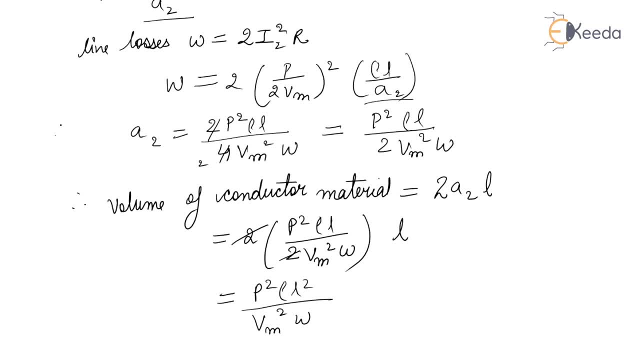 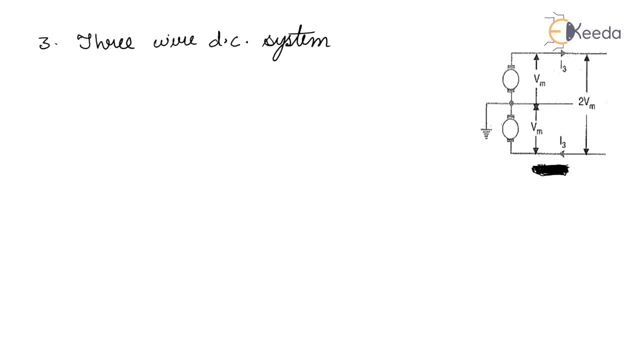 W Vm square is equal to A, So from this it is equals to W k upon four. now, volume of conductor middle required for three wire dc system. in this there are two outers and a middle or a neutral wire, which is odd. if load is balanced, current in the neutral wire is zero, so load current is equals to. 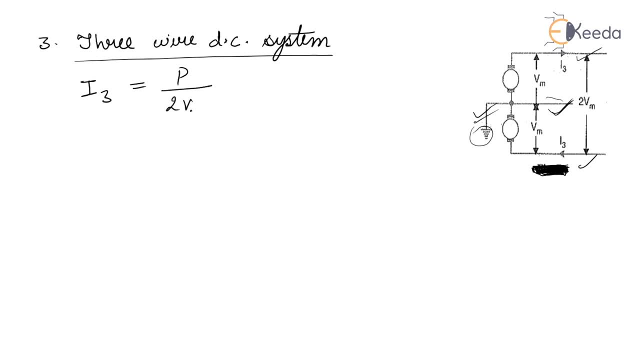 power upon maximum voltage. maximum voltage between the conductor is 2 vm and power to be transmitted is equals to p. again, if r is the resistance of each line conductor, then r is equals to rho l upon a3, where a is the area of the extension of the conductor. line losses is equals to: 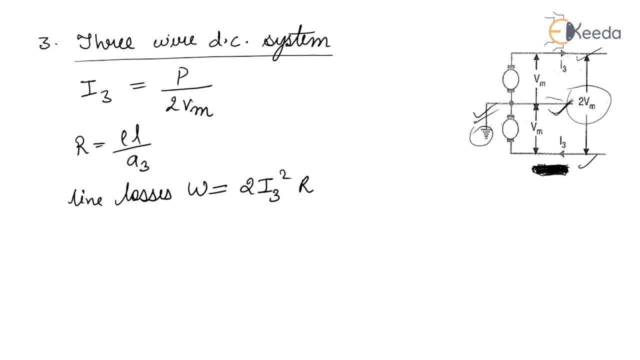 where i3 is power upon 2 vm and r is rho l upon a3. put the value of i and r now for volume of conductor metal required for three wire dc system is 2.5 area into length. so from this equation we have to find out the area. 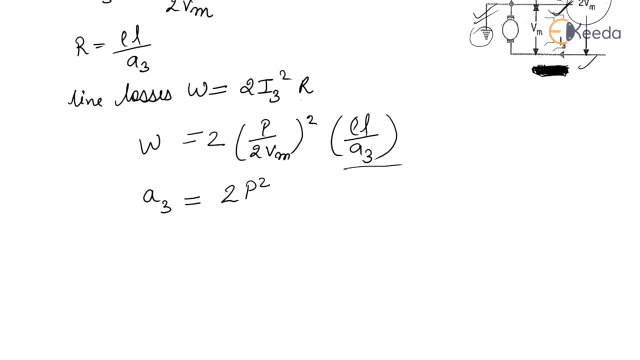 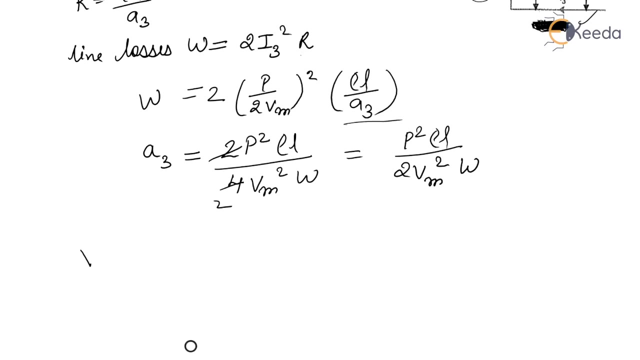 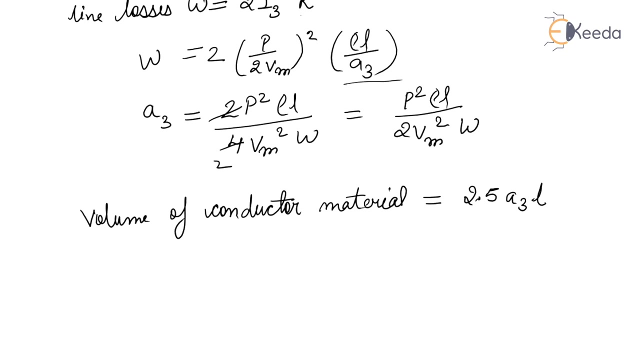 area is equals to 2 p square rho l upon 4 vm square w, which is equals to p square rho l upon now. volume of conductor material required for three wire dc system is equals to 2.5 area into length. assume the area of extension of neutral wire to be the half of the outer wire, that is, the. 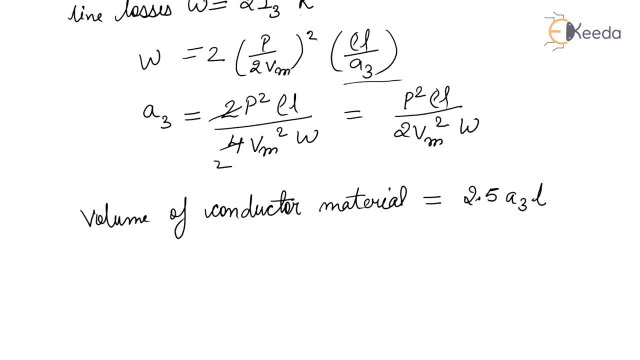 volume of the conductor metal required is equal to 2.5 area into length. put the value of area m square w in 2, L is equals to c, b is equal to 4 p square rho l upon w Vm2.. So from this equation we can write pi upon 16k. Hence the volume of conductor. 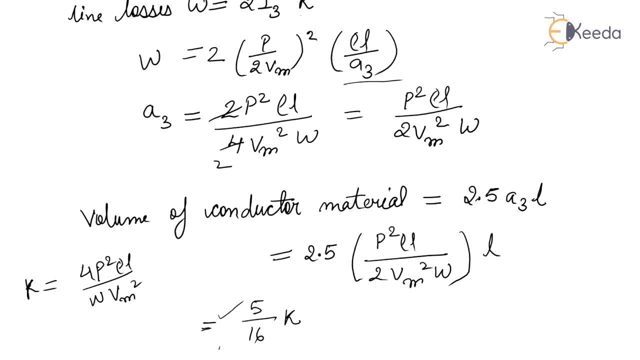 material required in this system is 5 by 16 times of what we required for 2 wire DC system with one conductor earthen- See the volume of conductor. material required in this system is 5 by 16 times of what we required for 2 wire DC system with one conductor earthen. 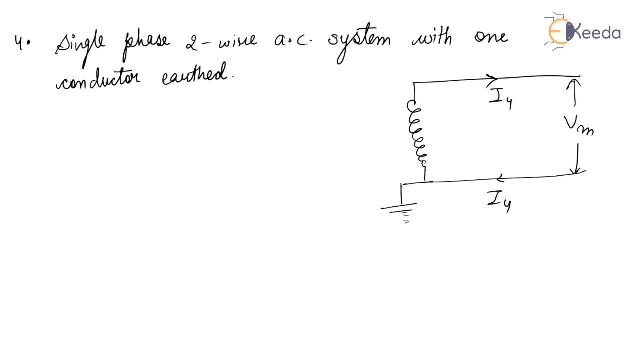 Now volume of conductor required for single phase 2 wire AC system. Now figure shows a single phase 2 wire AC system with one conductor earthen. Now. maximum voltage between the conductor is Vm, So Rm is value of voltage between them is Vm upon. 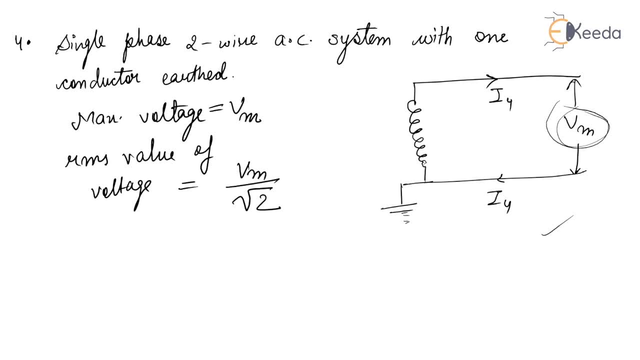 root. 2. Assuming load factor to be 4. Cos phi, the load current is equal to. for AC system it is equal to power upon maximum voltage, which is Vm upon root 2 cos phi. It is equal to Vm upon root 2 cos phi. So. 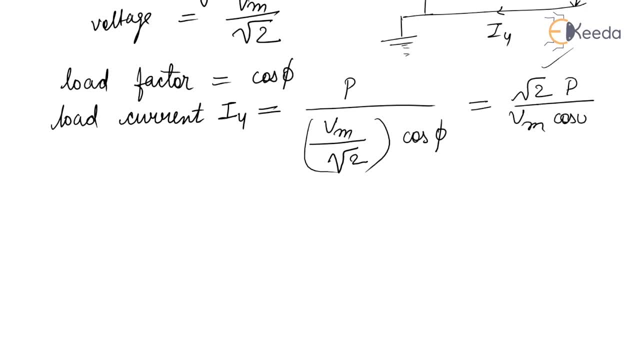 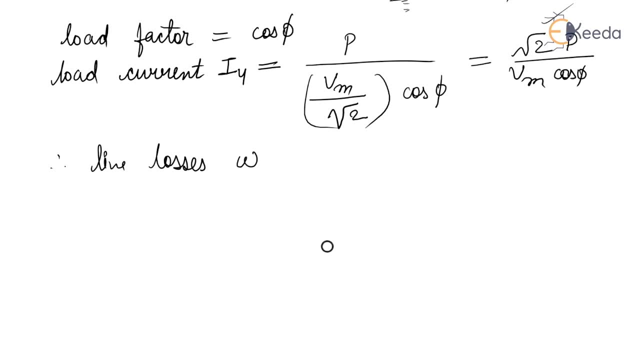 root 2P upon Vm upon cos phi- Now line losses- is equals to 2I square R. We know R is equals to rho L by A, where A is the exception of the conductor. Put the value of I and R through root 2P upon Vm upon cos phi, whole square into R is rho L upon A4 where A is the area. 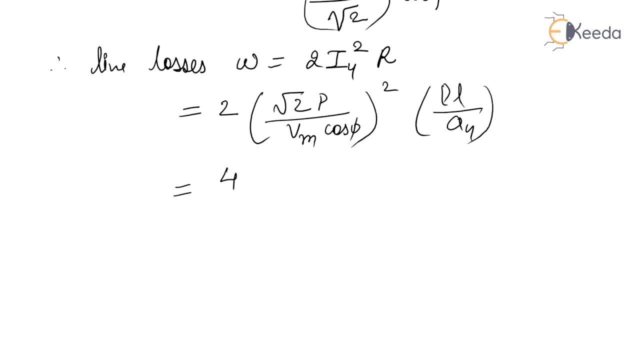 of the exception of the conductor, It is equals to 4P square rho L upon Vm square cos square phi A4.. Now we have to find out the volume of conductor material required for 2 wire AC system, which is 2 into area, into length. So from this equation, area is equals to 4P. 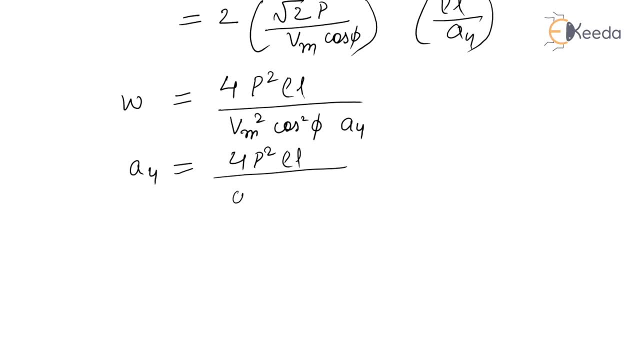 square rho L upon. therefore, volume of conductor material is equals to. volume of conductor material required is equals to 2 area into length. Now put the value of area which is 4P square Rho L upon cos square, phi W, Vm square, into L, It is equals to, Now, 4P square rho L square. 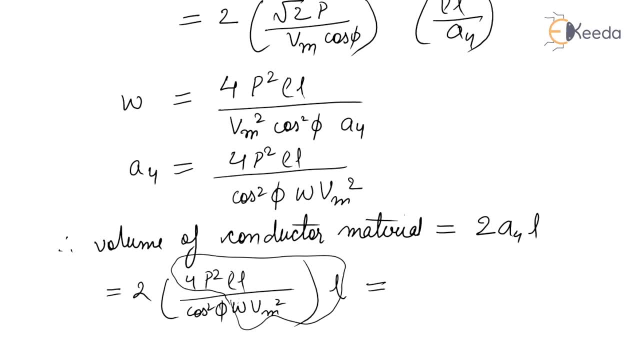 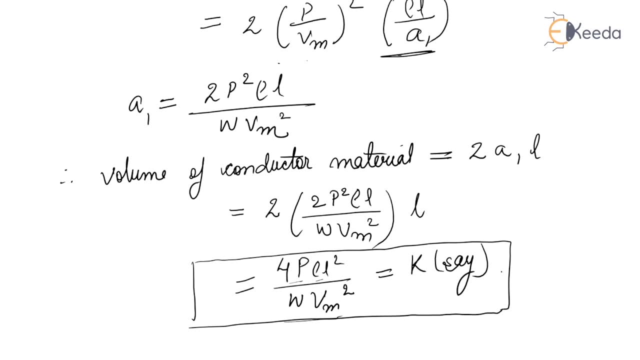 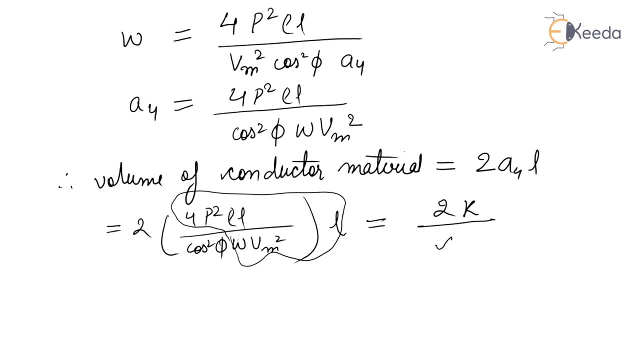 upon V Wm square is K. So 4P rho L square upon W Vm square is equals to K. So this equation is equals to 2K upon cos square phi. So volume of conductor material required in this system is 2 upon. 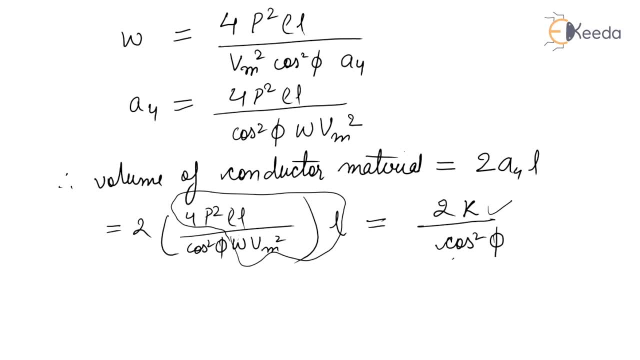 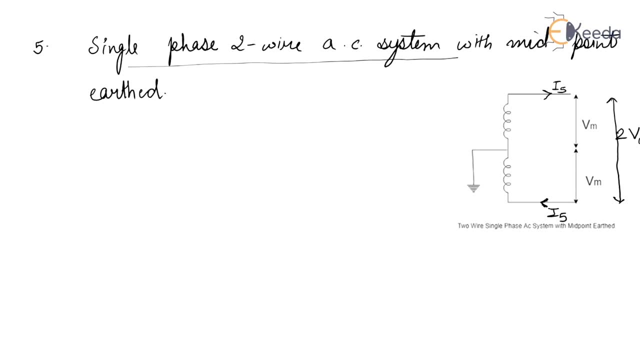 cos. square phi times. 2 wire DC system: 1 conductor earth. end Now volume of conductor material required for single phase 2 wire AC system with midpoint earth. Here figure shows the 2 wire single phase AC system with midpoint earth. Maximum bridge of both wires given between 2 wire is equals to 2 Vm. 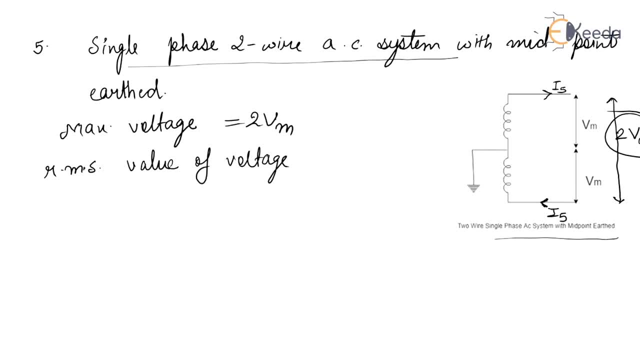 RMS value of voltage between conductors is 2 Vm by root 2, which is equals to root 2 Vm. Now load current current is equals to 2AAE, 2aE And MFV electric current current expansion is equal to RMSs value of current between 2shot highways. So these are the two solutions. 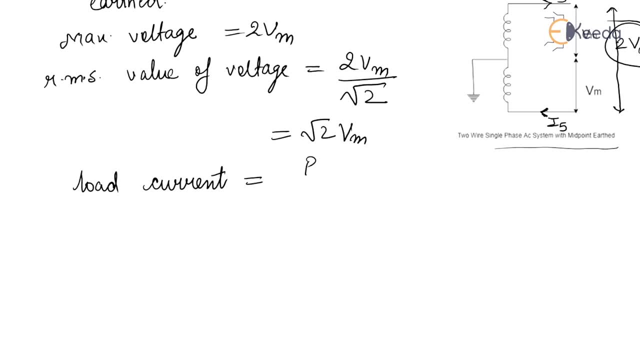 Now, with these two solutions, we are going to Down. We just want to measure current conservation of 2 Ross. all Now, with first figure, we are doing flow control, which is an effective method. we equals to power to be transmitted: P upon root, 2 Vm cos phi, where cos phi is the load power. 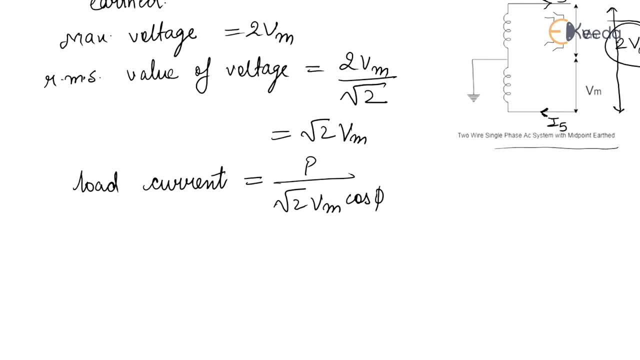 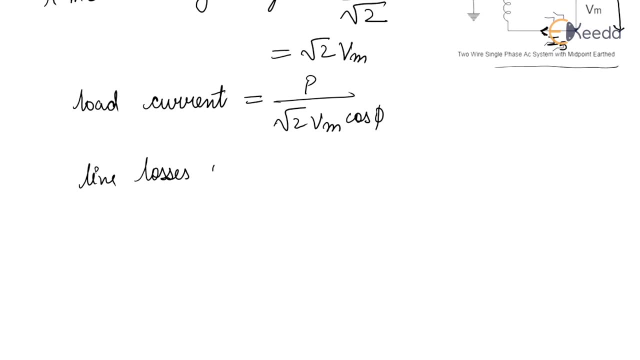 factor now line loss is: W is equals to 2 I square R. we know R is equals to rho L by A and I5 is equals to load. current I5 is equals to P upon root 2 Vm cos phi. put the value of I and R P upon root 2 Vm cos phi square into rho L upon A5, where A is the area of. 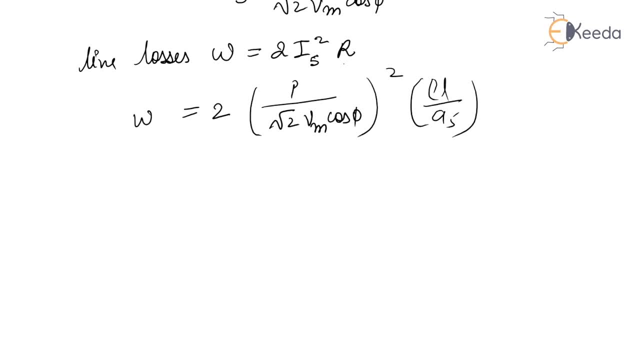 the x section of the conductor. so volume of conductor material required for single phase 2 IRC system is 2 area into length. so from this equation find out the area. area is equals to 2 P square rho L upon 2 P m square. cos square phi W, it is equals. 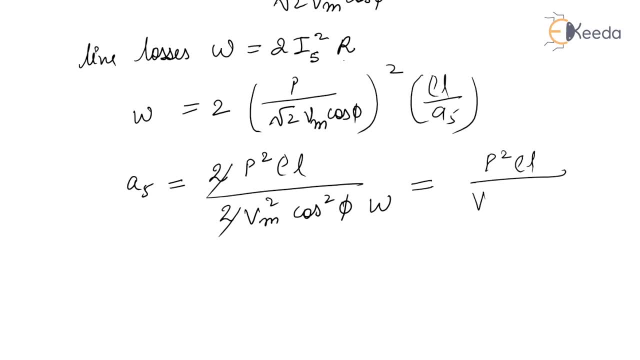 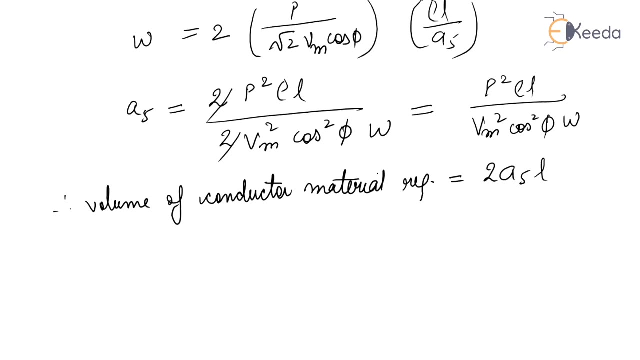 to P square, rho L upon Vm square, cos square, phi into W. now volume, therefore volume of the conductor is equal to P square, rho L into R water. it is goodbye D, we know. A is equals to P rho L square upon W Vm square, so it is equal to two area into length. I think we know. 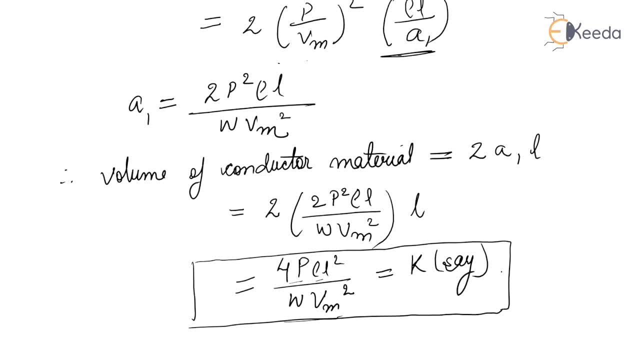 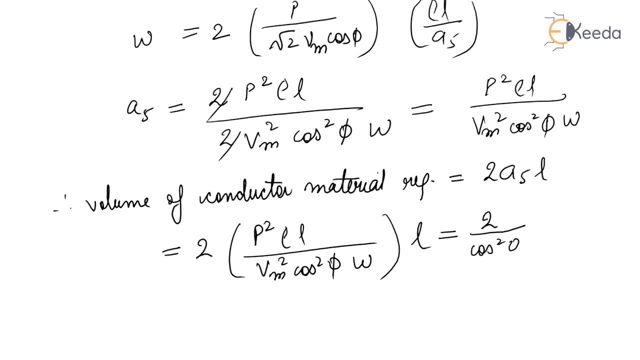 A is equal to two area into length. A is equal to R L divided by R, but there are four PE R M square per A is equal to 3 RL squared divided by R. L squared divided by R. Vm squared: 2 upon cos square, pi p square, rho L square upon WVM square. 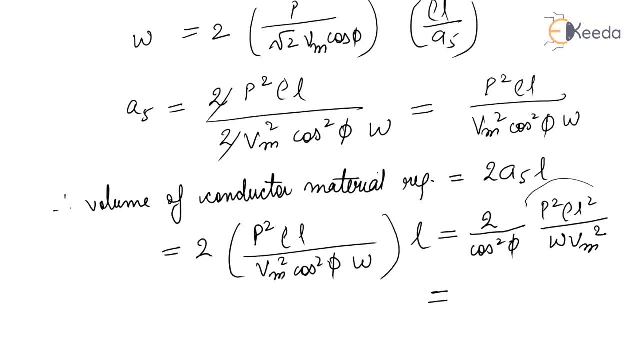 It is equals to k upon 2 cos square pi, Because we know 4 upon p square, rho L square upon WVM square is k, So we can write this as 2 upon cos square pi into 1 by 4.. So it is equals to k upon 2 cos square pi. 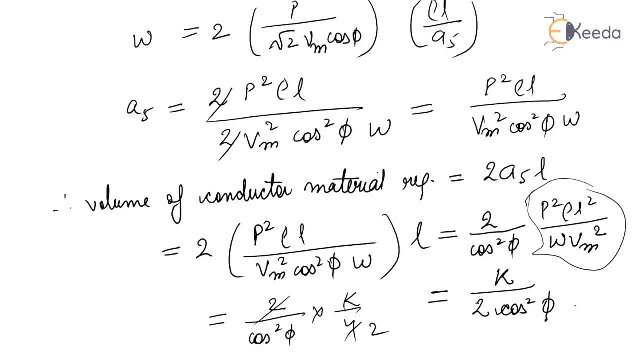 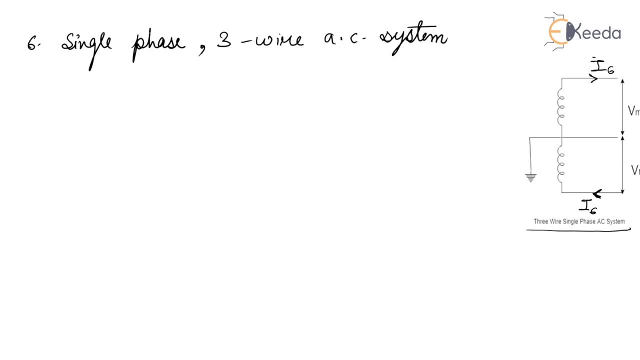 So we can see that 1 by 2 cos square pi times the 2 wire DC system. Now, volume of the conductor material required for single phase 3 wire AC system. Figure shows the 3 wire Single phase AC system. 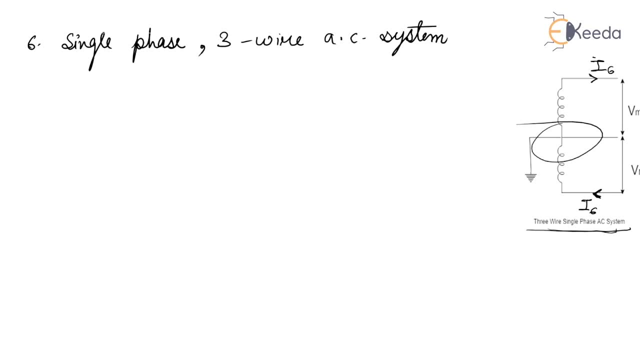 If load is balanced, current through third wire is neutral, So the maximum voltage is equals to 2 Vm RMS value of voltage between conductor is 2 Vm by root 2, which is equals to root 2 Vm. Power factor of load is cos 5.. 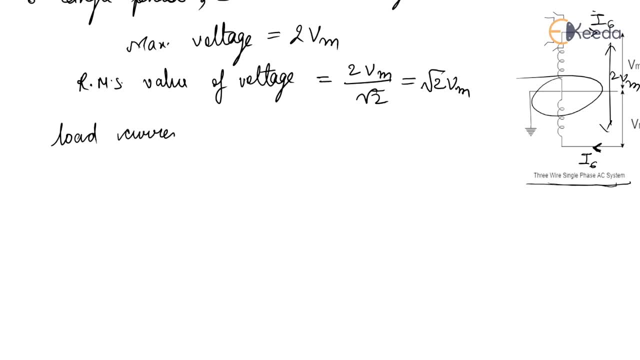 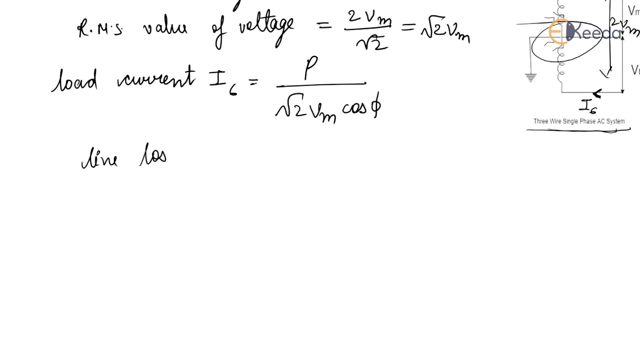 Then load current. So load current Is equals to power to be transmitted upon root: 2 Vm cos 5.. So load current Line losses is equals to 2 I square R, where R is the resistance of each line conductor, which is rho L by A. 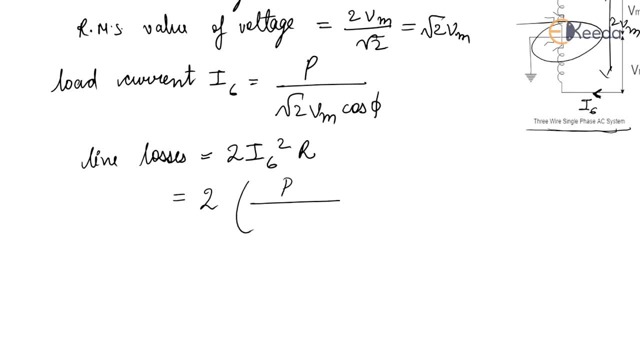 So put the value of I and R Power upon root 2 Vm cos phi, whole square R is rho L upon A6, where A is the area of the X section of the conductor. So volume of the conductor material required for 3 wire AC system is: 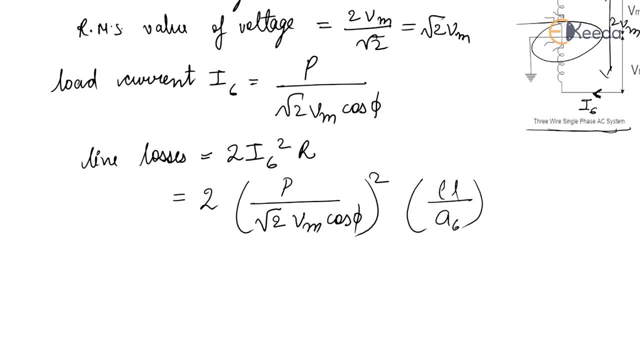 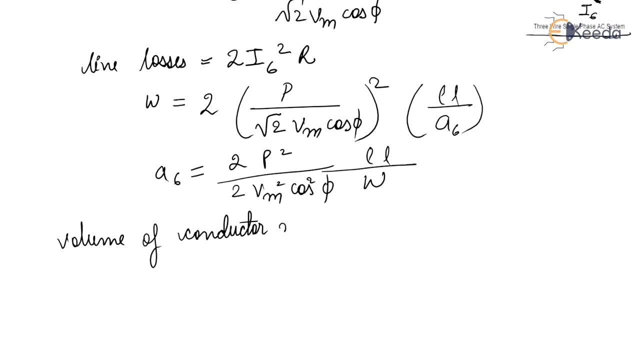 2.5 area into length. So from this equation we have to find out the area which is equals to 2 P square upon 2 Vm, cos, phi, rho, L upon W. Now, volume of conductor material required is equals to 2.5 area into length. Put the value of area. 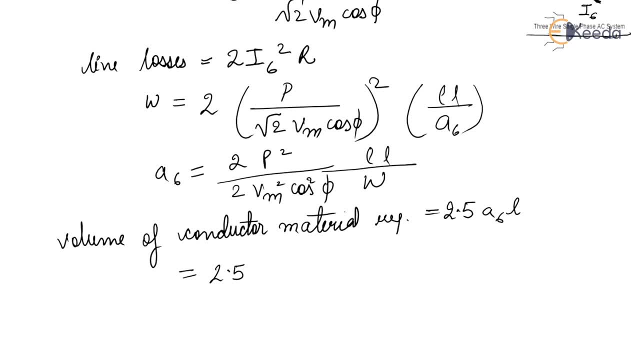 V is equal to 2.5 area into length. So from this equation we have to find out the area. we have to assume the area of X section of the neutral wire to be the half of the outer wire. So 2.5 area into length. 2.5 area is 2 P square. 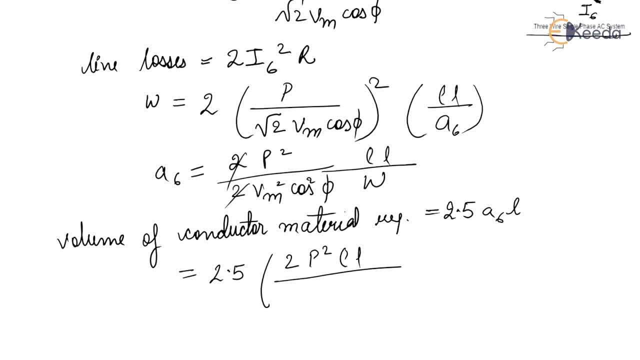 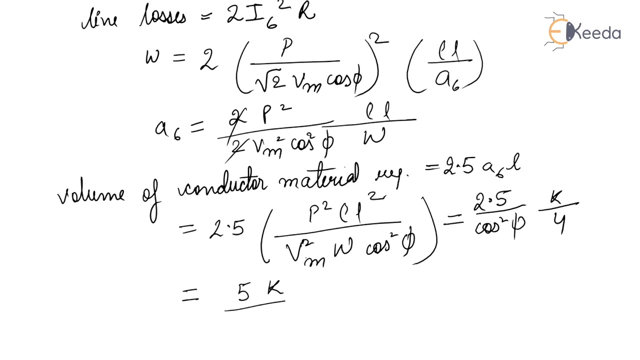 root L upon To-To cancel. So P square rho L upon V square M W cos square phi into L. So we know 4p square rho L square upon Vm square W is equals to k. So this is equals to 2.5 cos square, pi k by 4, which is equals to pi k upon 8 cos square. 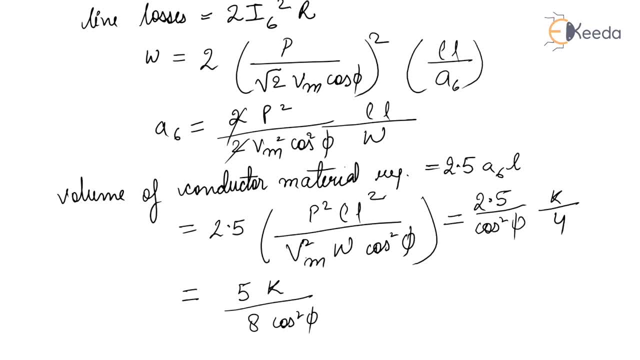 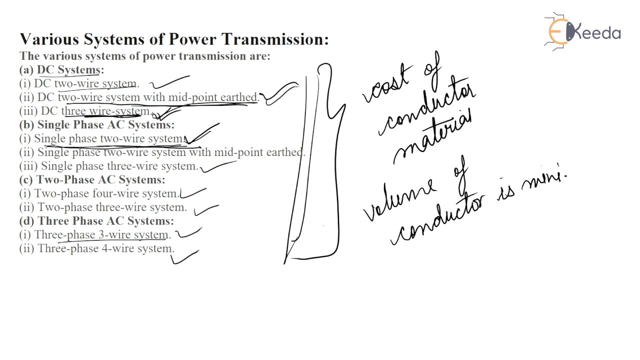 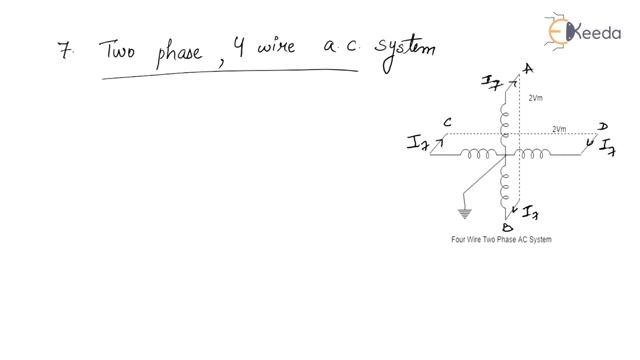 pi. Hence the volume of the conductor material required in this system is pi by 8 cos. square pi times the 2 wire DC system with one conductor earth. Now volume of conductor material required for 2 phase 4 wire AC system, See: maximum voltage between A and B is equals to 2 Vm. 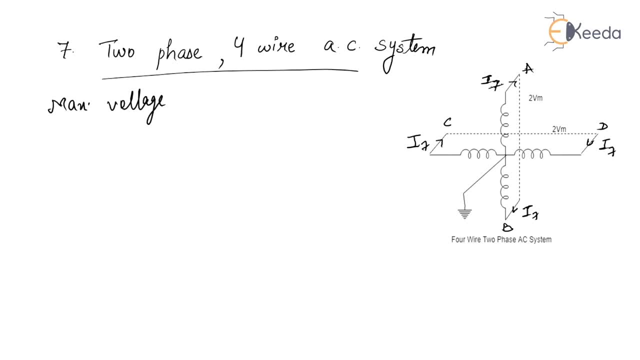 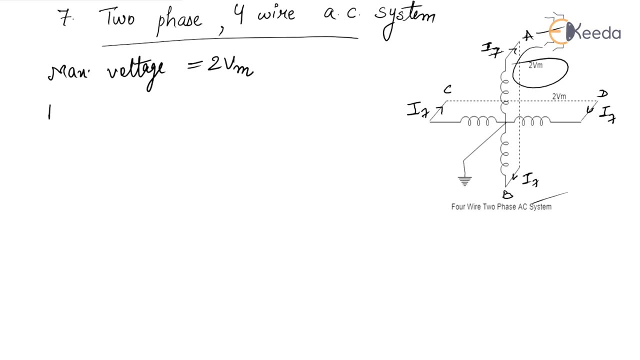 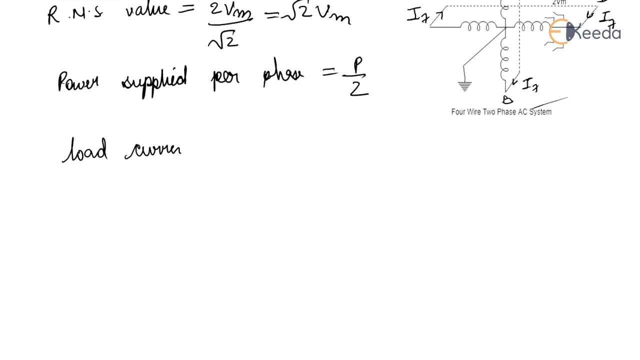 RMS value of voltage is equals to 2 Vm by root 2, which is equals to root 2 Vm. Now, power supplied per phase is equals to T by 2.. Assuming power factor of the load is equals to cos phi, then load current is equals to. 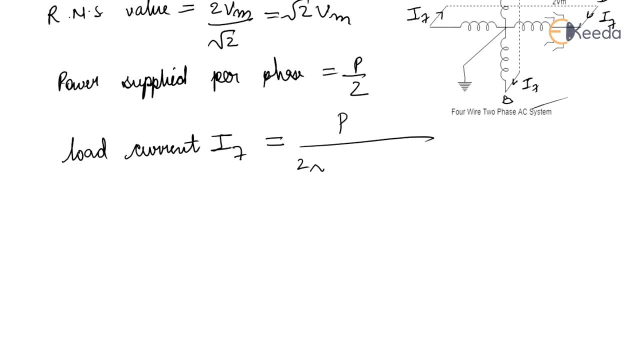 T by 2 root 2 Vm cos phi, Then line losses is equals to: for 4 wire AC system is equals to 4.5 Vm by root 2 Vm cos phi. We know R is equals to rho L by A, where A is the area of the x-section of the conductor. 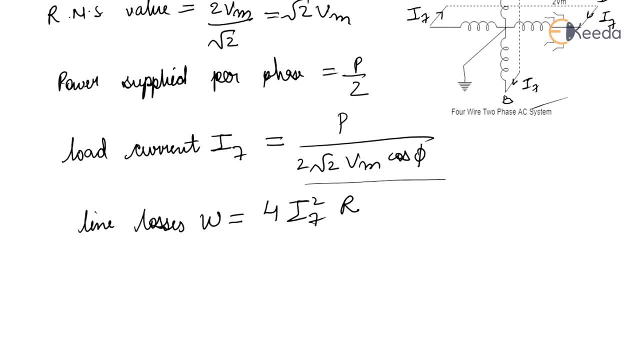 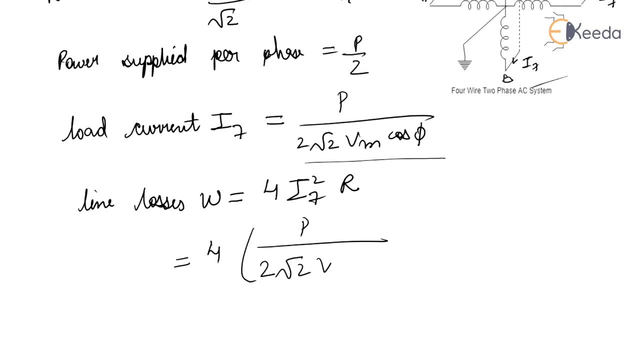 and current I7 is p upon 2 root 2 Vm cos phi. Put the value of I and R for p upon 2 root 2 Vm cos phi whole square into rho L by A, where A is the area of the x-section of the conductor. 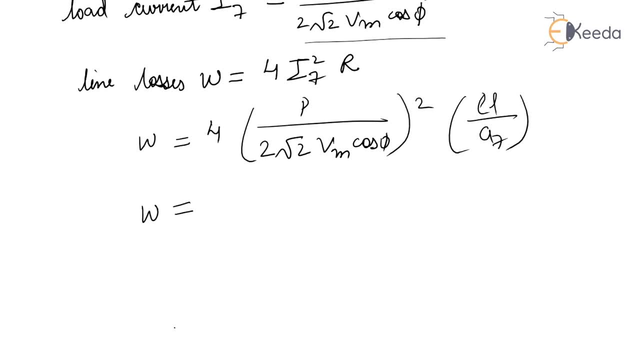 Now W is equals to 4 p square upon 8 V square cos phi rho L by A. Now volume of conductor material required for 4 wire AC system is 4 area into length. So from this equation find out the area. Now volume of conductor material required for 4 wire AC system is 4 area into length. 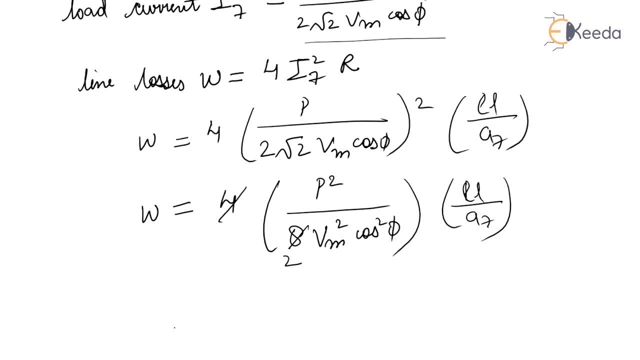 So from this equation find out: the area Which is equals to area is equals to p square rho L upon 2 V square cos phi W Which is equals to area is equals to p square rho L upon 2 V square cos phi W. 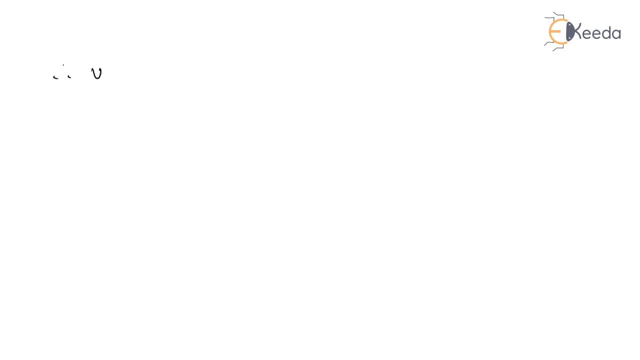 Therefore, volume of conductor material required for 4 wire AC system is 4 p square rho L by A, where A is the area of regular root V square, This is equals to 4 p square. rho L square upon 2 W e q2 cos ϵ W. This is equal to four e to the alive p square. rho l square upon 2 w vs cos phi, Wb, cos2 profit. 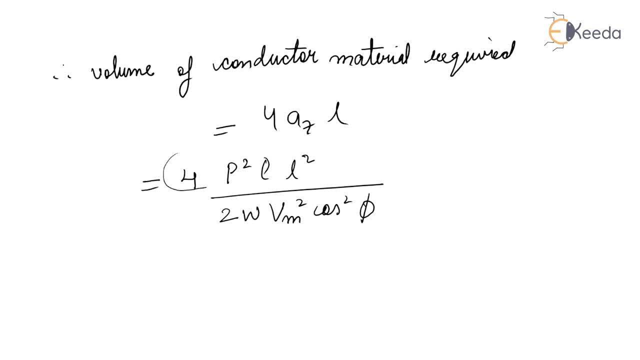 cos square phi. We know 4p square, rho l square upon wvm square is equals to. so this is equals to k upon 2 cos square phi. Hence the volume of the conductor material required in the system is 1 by 2 cos square phi times the required in a two wire DC system with 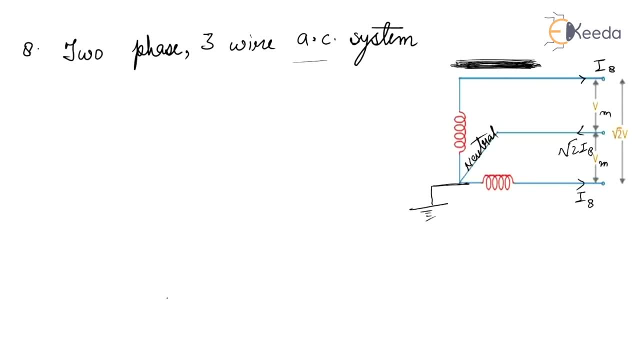 one conductor. R Figure shows the two phase three wire AC system. The third or the neutral wire is taken from the junction of two phase winding whose voltage are in quadrature with each other. Obviously each phase transmits one half of the total power, so the rms voltage between outgoing 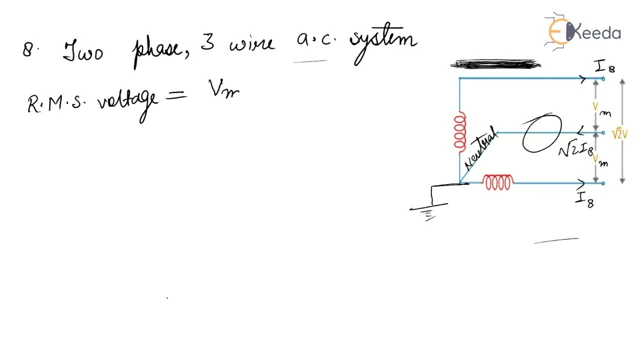 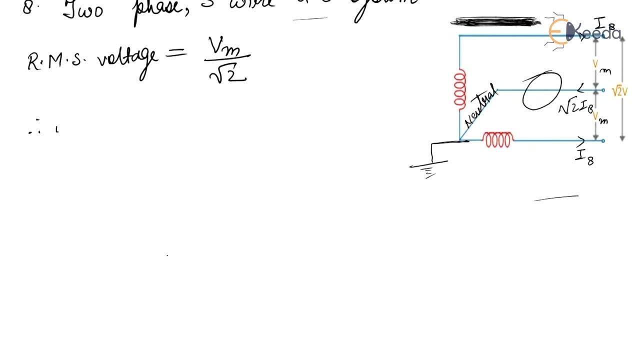 and neutral is equals to vm by root 2 and power to be transmitted is equals to p by 2 per phase. Therefore, current in each outer is equal to p by 2 upon vm by root 2, cos phi and current in neutral wire. this neutral wire. 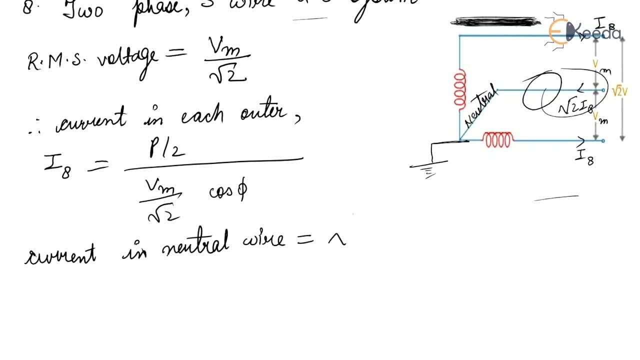 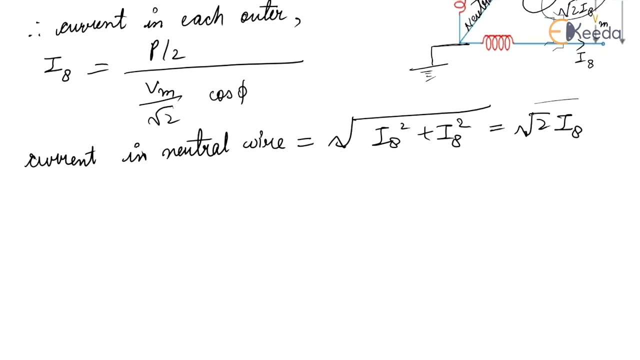 is equals to under root i square plus i square, which is equals to root 2. i Assume current density to be constant. area of extinction of neutral wire will be root 2 times of either of the outers. Therefore, resistance of neutral wire is equals to R. 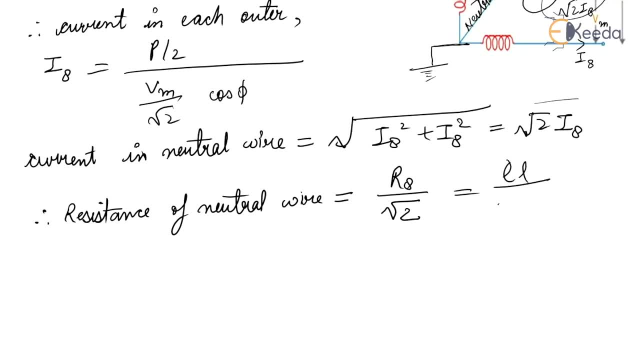 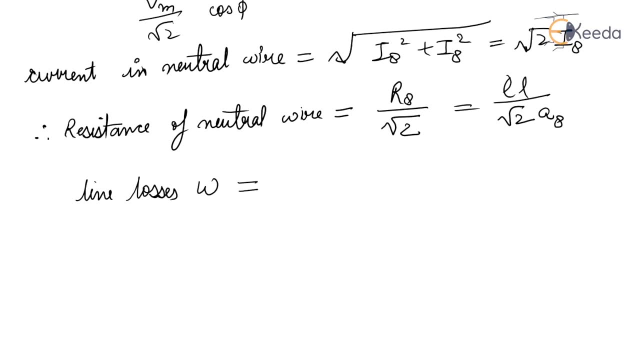 by root 2, where R is rho L by 8.. Line loss is: W is equals to 2 I square R plus neutral wire root 2 I square R. This is equals to I square R, 2 plus root 2.. Now put the value. 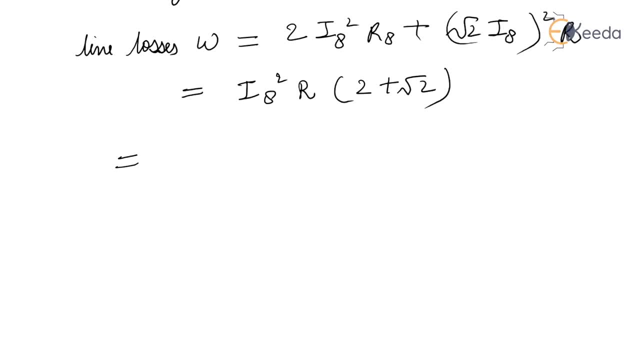 of I and R, which is equals to P square rho L upon 2 A V square cos square phi 2 plus root 2.. Now volume of connecting material required for two phase three wire system is equals to, for outer wire, 2 area into length plus neutral. 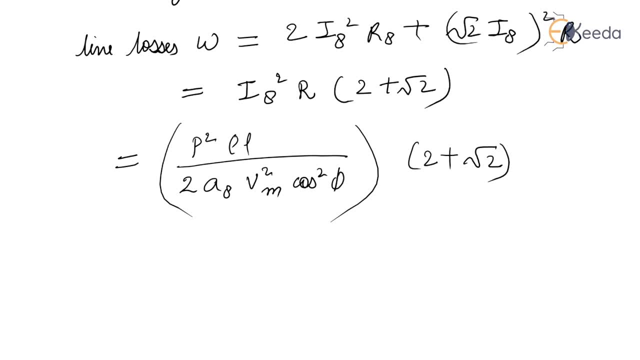 wire root 2 area into length. So find out the area from this equation which is equals to P square rho L upon 2 W V square cos square phi 2 plus root 2.. Therefore, volume of connecting material required is equals to 2 area into length plus root 2. area into length which 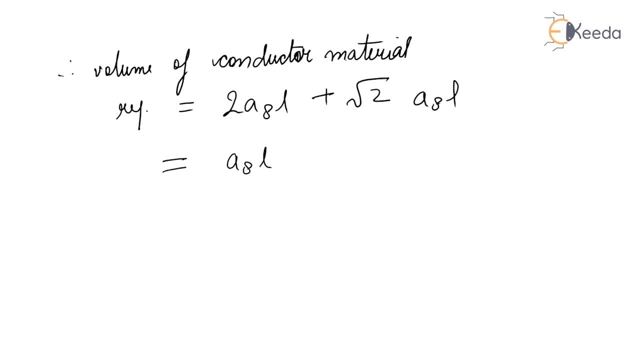 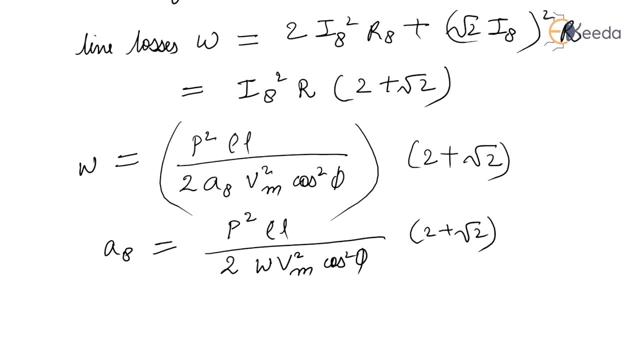 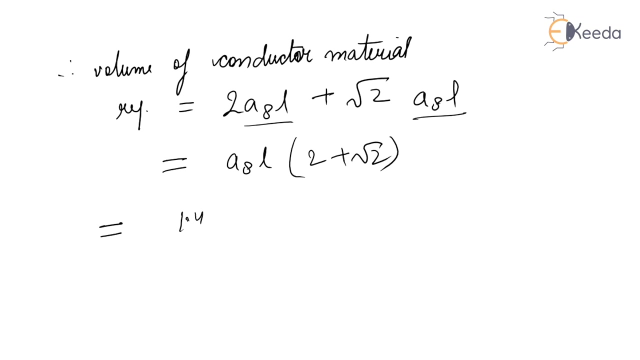 is equals to a common A and L. Put the value of area, this and the volume of connecting material required, you get 1.457 upon cos square phi times K. Hence the volume of the connecting material required in this system is 1.457 by cos square phi times the required in a two wire DC system with one conductor. 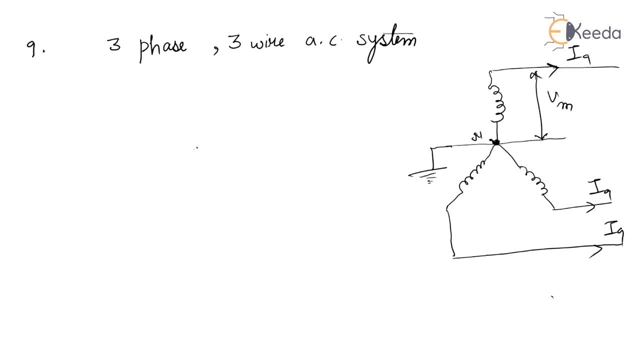 odd. Now the volume of the connecting material required for three phase three wire AC system. This system is universally adopted for transmission of electrical power. Figure shows the three phase three wire star connected system. This is the neutral point N, which is odd. So Rms voltage. 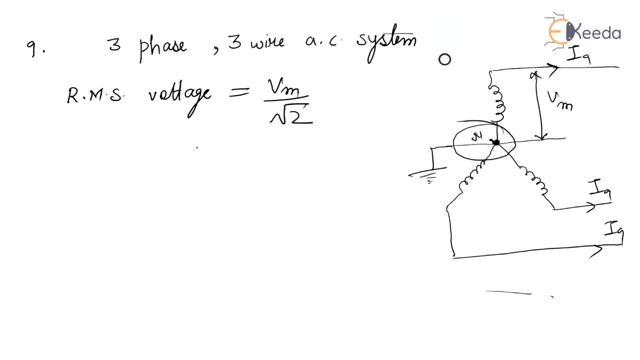 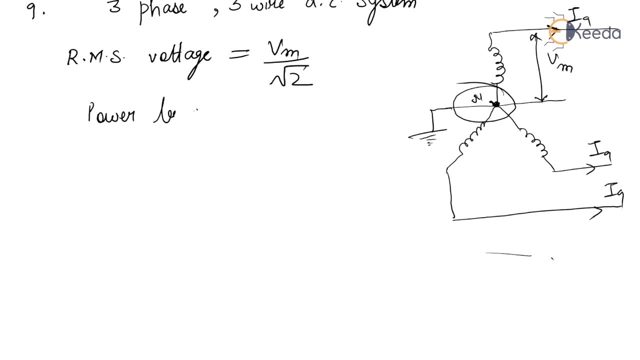 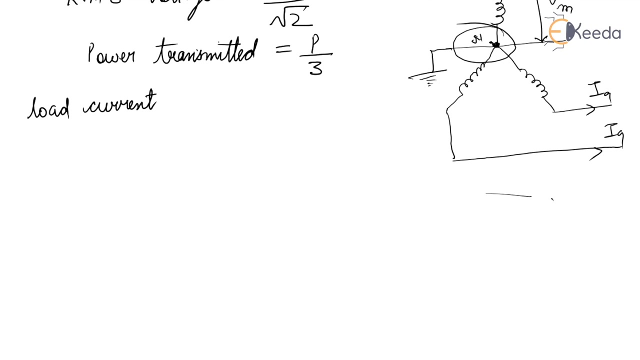 per phase is equals to Vm by root. 2.. Power transmitted per phase equals to P by 3.. The radical of this band will be of food form. The particular factor which is equal to weight power will be of C. Now, load current per phase is equals to P by 3 upon Vm by root. 2 cos phi, which is 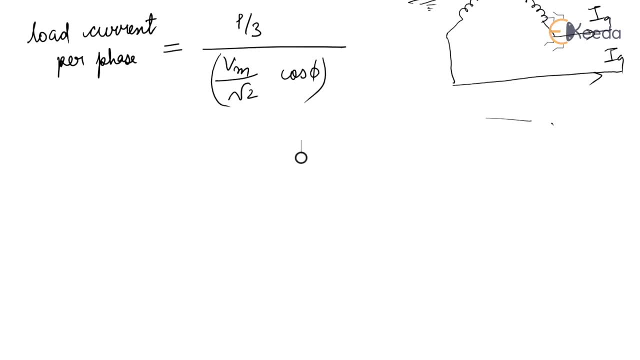 equals to root 2 P upon 3 Vm cos phi. Now line losses. W is equals to: for 3, wire 3, I square R. We know the value of I, Which is root 2 P upon 3 Vm cos phi, and R is Rho L by A Put the value of I and R P. 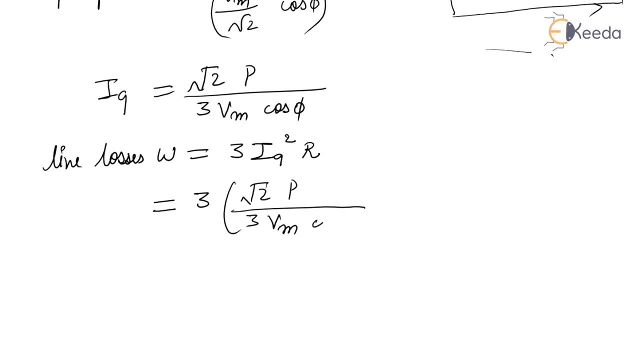 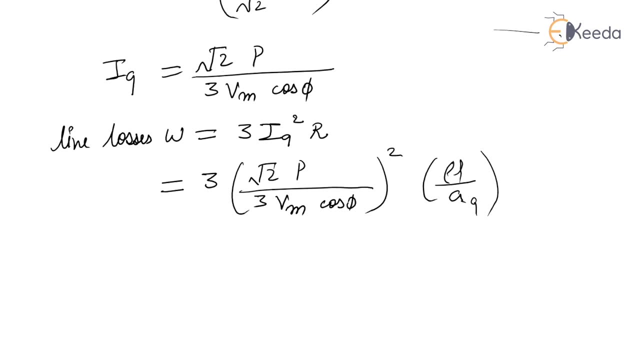 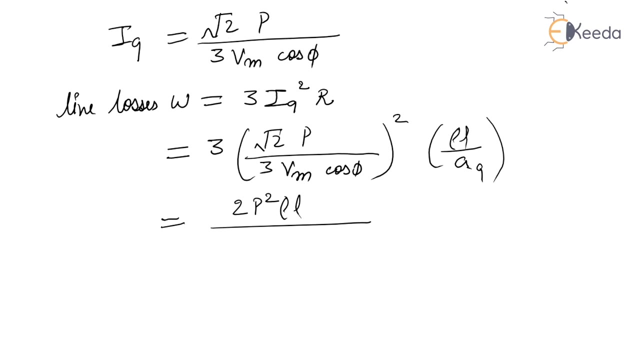 root 2 P upon 3 Vm cos phi square into Rho L by A, Where A is the area of the section of the conductor. This is equals to 2 P square Rho L upon 3 Vm cos phi. Now, volume of the conductor. material required for 3 phase 3 wire system is 3 area. 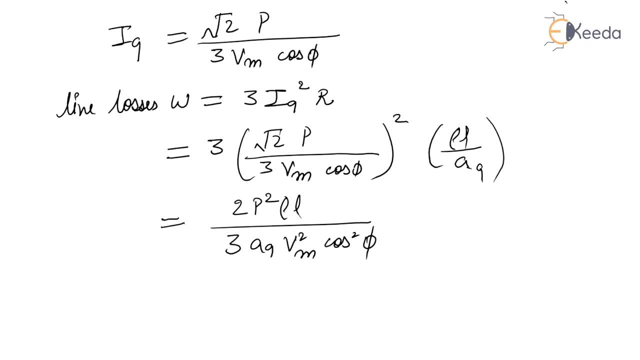 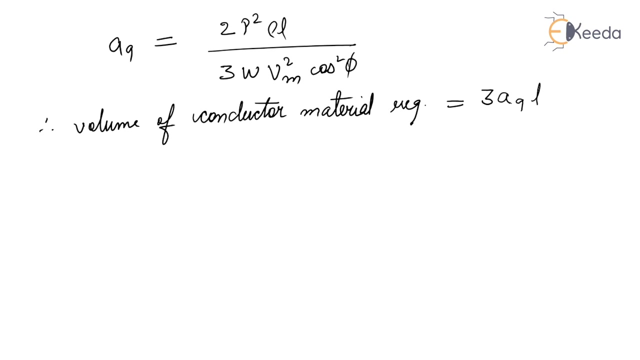 into length. So from this equation find out the area. So area is equals to 2 P square, Rho L, 3 W V square, cos phi, 3 W V square, cos phi. Therefore volume of conductor material required is equals to 3 area into length. Put the value of area 3, 2, 3 2 P square, Rho L upon 3 W V square. 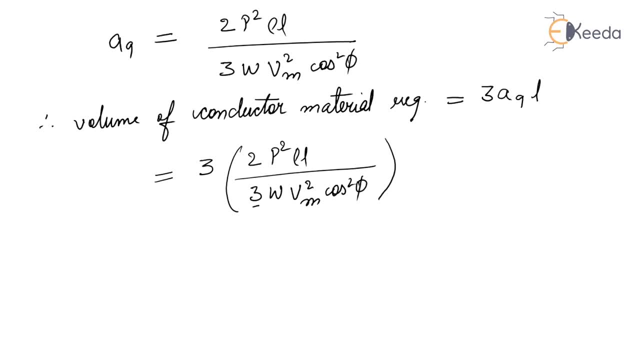 cos phi 3 W V square. cos phi into L L square. We know 4 P square, Rho L square. W V square is equals to K, So this is equals to 2 upon cos phi K by 4.. So this is equals to 0.5 upon cos phi. 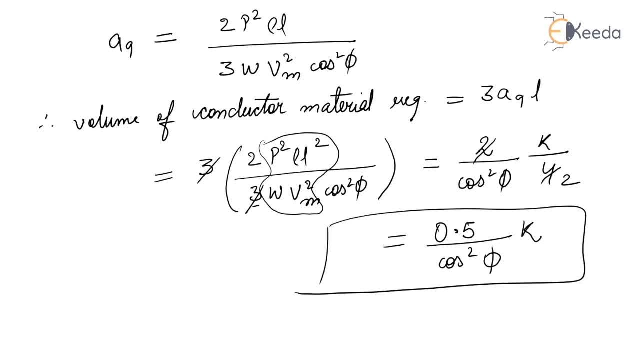 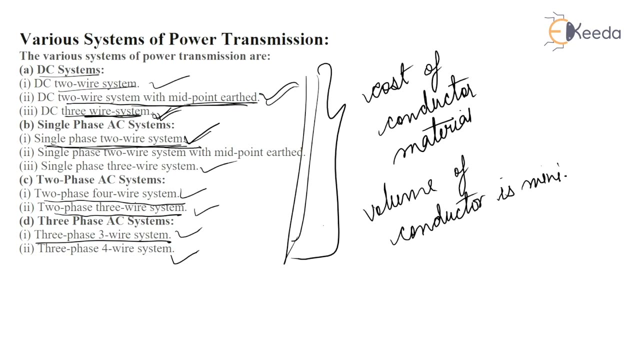 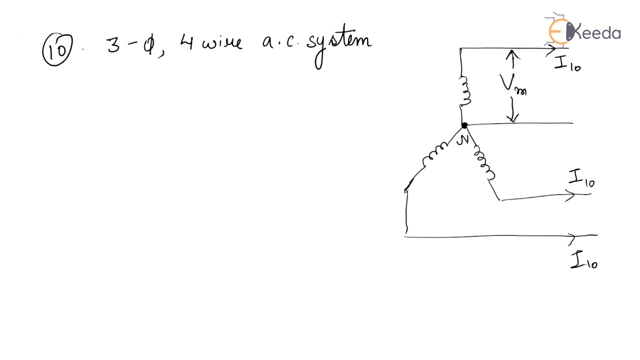 times that required for 2 wire DC system with 1 conductor R. So volume of conductor material required for 3 phase 4 wire AC system. Figure shows the 3 phase 4 wire AC system. In this case, 4th wireless wire is taken from. 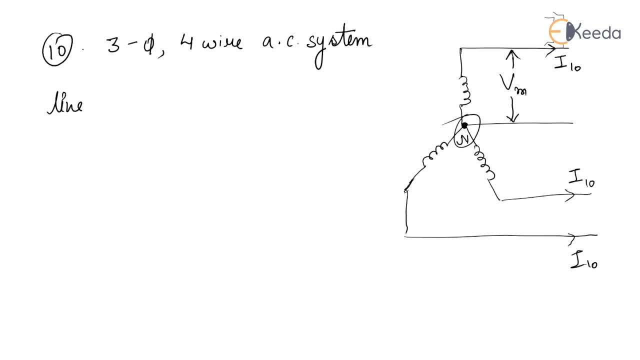 the neutral point. the line loss is: w is same as in 3 phase 3 wire, that is, 2 t square rho l upon 3 k, 10 v square, cos square 5.. Now volume of conductive metal required for 3 phase 4. 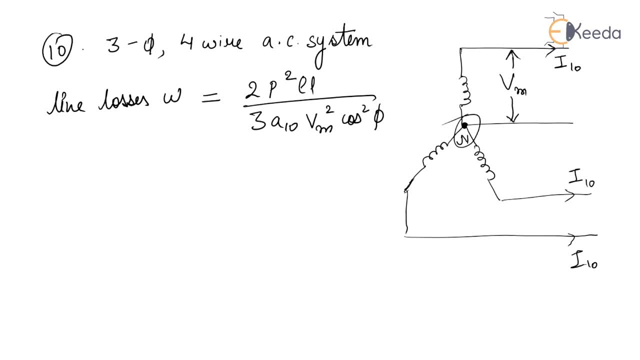 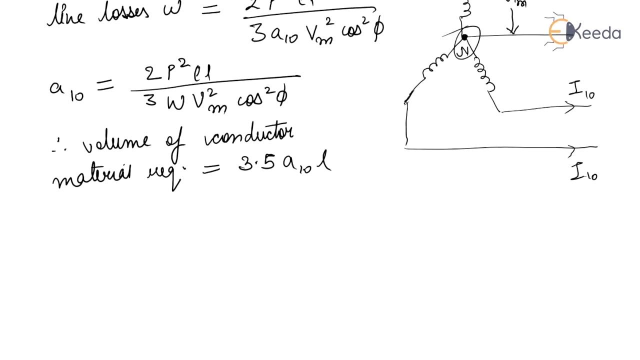 wire AC system is equals to 3.5 area into length. So from this equation find out the area which is equals to 2 t square, rho l upon 3 w v square, cos square 5.. Therefore, volume of conductor material required is equals to 3.5 area into length. Put the value of area which is equals to 3.5 2 t square. 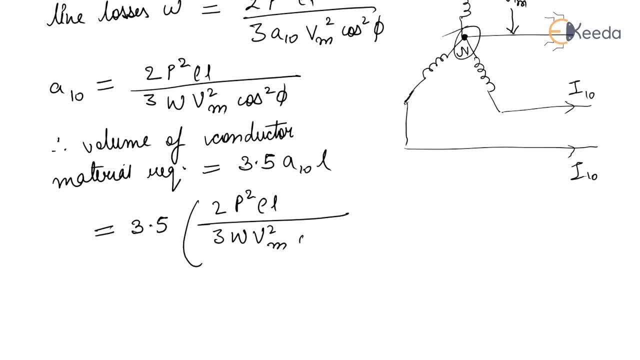 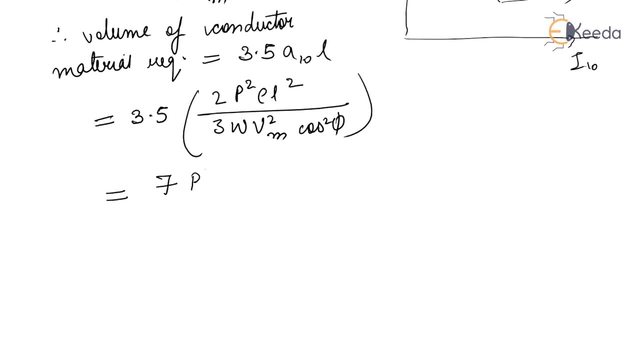 rho l upon 3 w v square, cos square 5 into l l square. Now we know: 4 t square rho l square upon w v m square is equals to k. This is equals to 7 t square rho l square upon 3 w v square, cos square 5.. We can write this as: 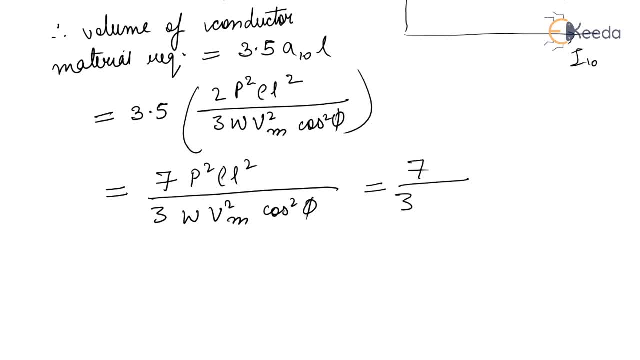 7 upon 3 cos square 5, because we know 4 t square rho l square upon w v m square. is스가 equals to kax t square rho. laud cheek upon w ligne 38.5 k, Talking about mb j, is equal to 3.5 area. into l Quad square 4 into m squared. you can write: 3.5 u square. rho l square equals to k r p square. rho l square upon w v square equals to solution P. star 3 is equals to 1 into m of R square. rho l square, double general when disputeών. 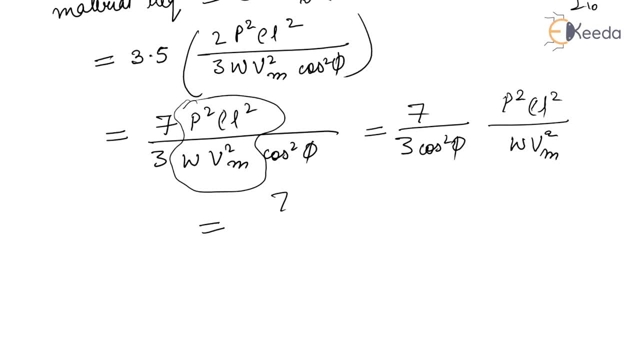 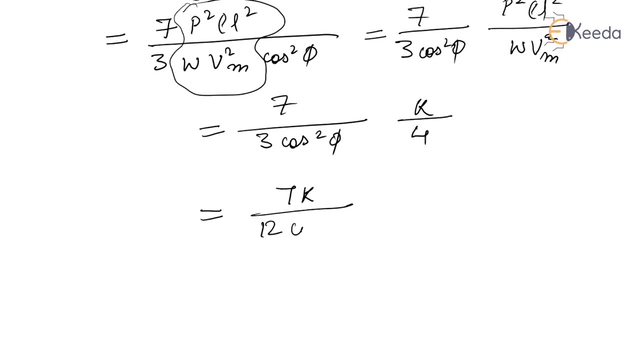 square, This is equal to 7 upon 3 cos square k by 4, which is equal to 7k upon 12 cos square pi. Hence, the volume of conductive material required for this system is 7 by 12 cos square, 5 times the required for 2 wire DC system with 1 conductor earth. Thank you,